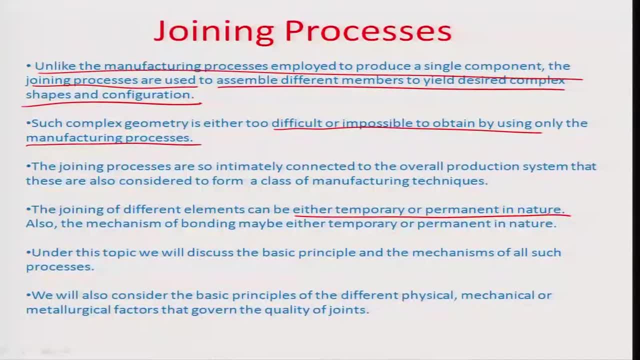 something like, let us say, solid state welding, where there are two components which are pressurized very close to each other So that there is some kind of a bond formulation between them may be easily recorded as a permanent joining process. So that is how you classify and 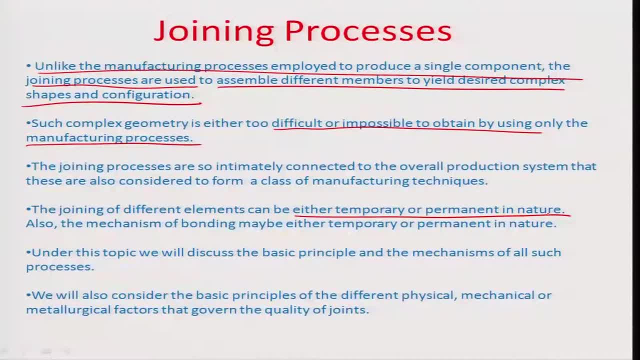 this is the first classification of all the different joining processes, So we will basically describe some of the principles and the mechanisms in all such processes and with the physical or mechanical point of view, and also some of the metallurgical viewpoints which emerge while studying such joining processes would be treated in this. 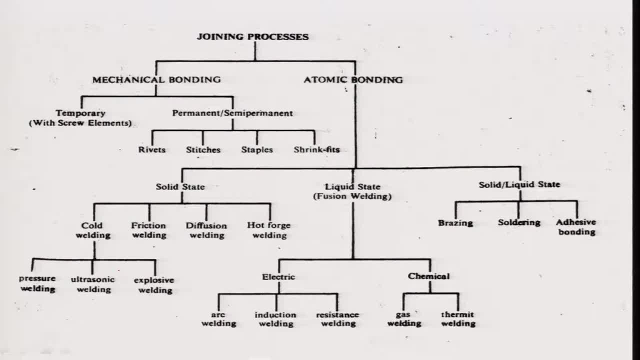 particular area. So let us look at a classification schematic of the various joining processes. So generally, joining process can be classified into mechanical bonding and atomic bonding. Mechanical bonding could be again classified into more permanent or semi-permanent kind of joints and a temporary with screw elements, for example, as I just mentioned earlier. 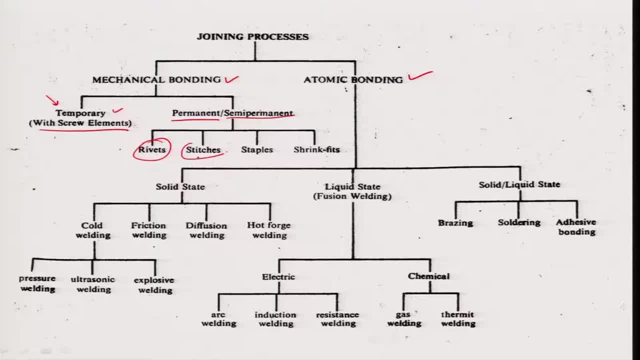 In the permanent, semi-permanent category, there can be riveting, there can be stitching between two surfaces or stapling between two surfaces, or even shrink fits sometimes, which ensures that So there can be some kind of semi permanency between the joints. that means if, for example, 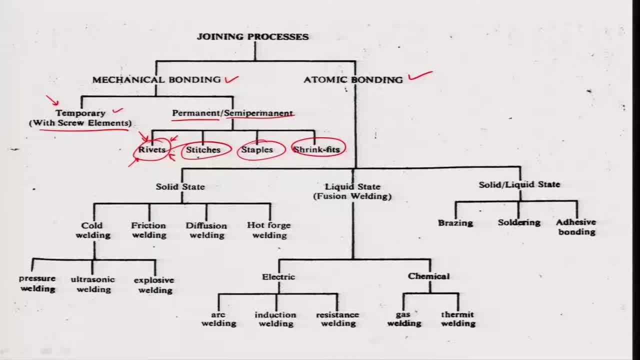 in the case of rivets, without destroying the rivet or without breaking the rivet head open, you cannot really undo the joining process. So it is some kind of a semi-permanent intermediate kind of a joining So in. so therefore, that is how semi permanent joints can be interpreted. 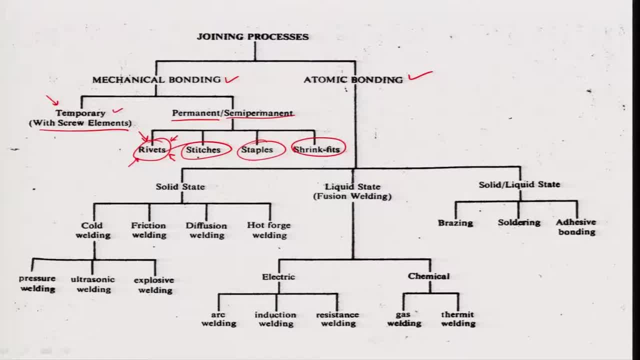 Now the other type of joining happens more on atomistic basis, where you can have two crystals, for example. were two different materials, for example, taken so close to each other by virtue of pressure and some deformation that there is some kind of a cold weld which 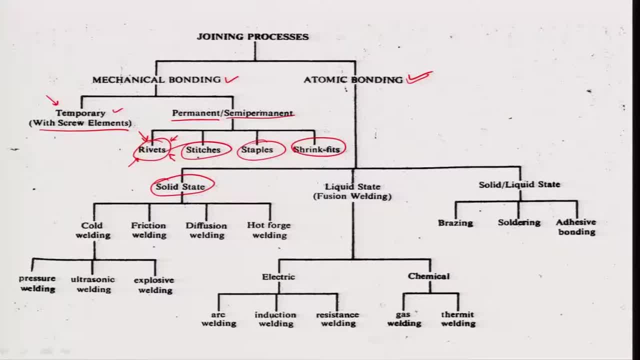 is formulated within the two surfaces. So such surfaces are, or such kind of bonding is also known as solid state bonding. there can be again liquid state bonding, and bonding can also be in solid and liquid state. I will just explain some of the solid state bonding. 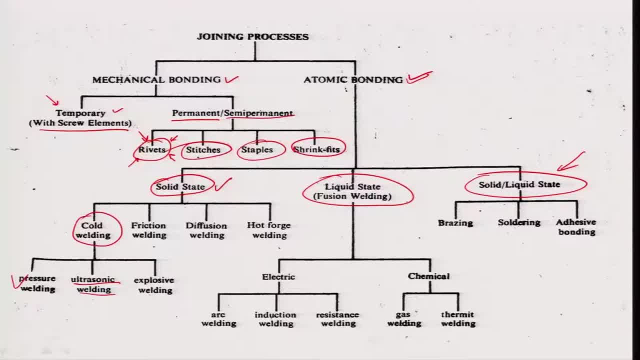 So one of the examples, for example, you know, could be like cold welding, where I, two members, two metallic plates, for example, are brought very close to each other and applied with certain pressure So that the distances between the surfaces become almost equal to that of 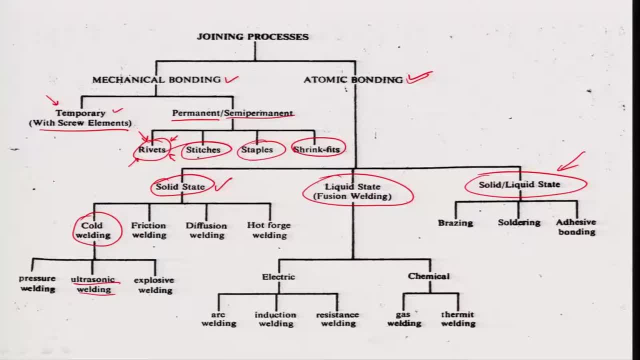 a grain boundary. So there is automatically increase in the inter atomic forces because of, probably, the electrons of one set of atoms attracting the getting attracted by the nucleus of the other set of atom. but that close proximity or close distance between the surfaces need to be coming for this kind of a bonding to take place. 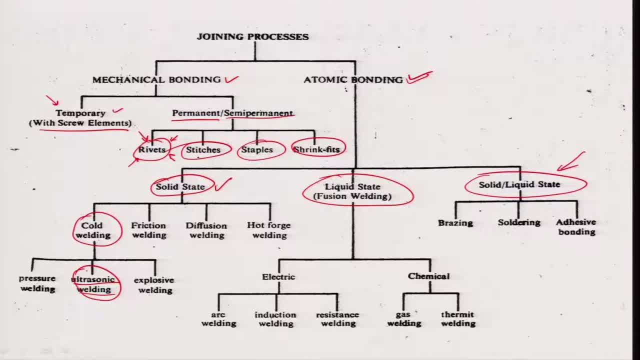 There can be again cases of ultrasonic welding, where you vibrate one of the components, one of the members, at an ultrasonic frequency So that you can again introduce proximity between the members in a manner So that there is a solid state bonding which takes. 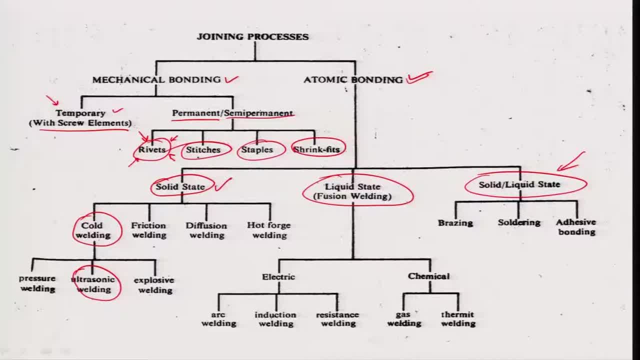 place So you can actually use an electric arc where what you normally do in arc welding, and there is arc established between an electrode and a surface which is very high power and high power consuming And it generates a stream of electrons which completely melts the parent. 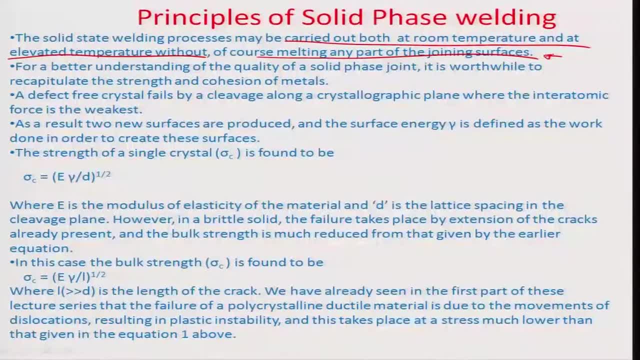 are surfaces which have solid, which are solid surfaces, they do not lose their integrity. and you know you can basically apply pressure as well as heat here to perform the welding. So for a better understanding of the quality of the solid phase joint, it is worthwhile. 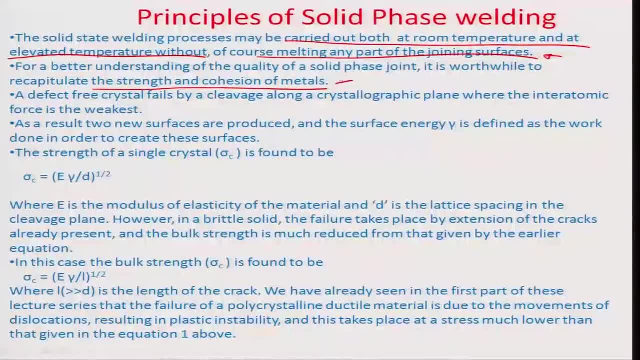 to recapitulate the strength and cohesion of metals. So a defect free crystal normally fails along a sort of a crystallographic plane where the inter atomic force is the weakest. So that is how there is a development of 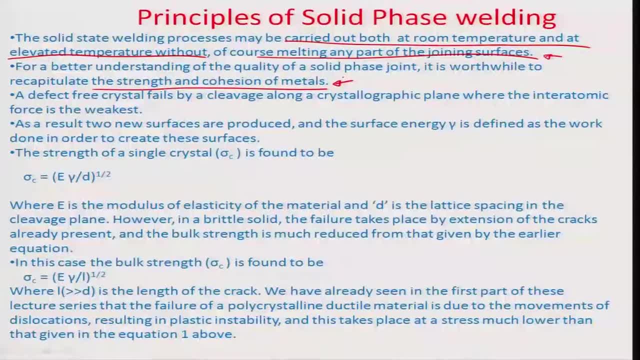 a crack. So wherever there is a case where the inter atomic force is the low, lowest value, and supposing you are now putting the object to a tensile strength, the failure would happen from that area where the bond between the materials is the weakest. 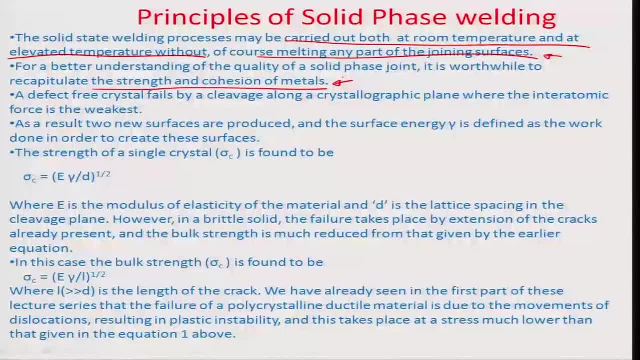 find as the work done in order to create those surfaces which you are doing externally. 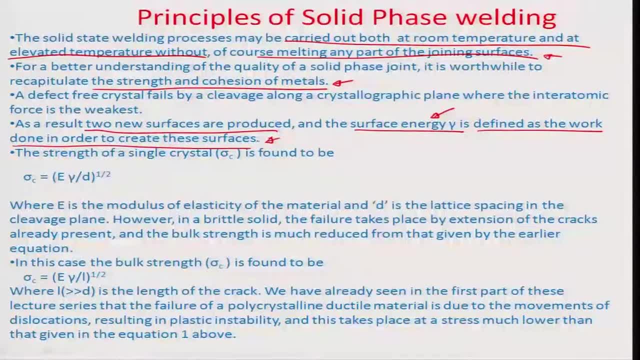 Obviously you are pulling the material to get this crack initiated or get this- you know- fissure initiated between the material. So whatever energy you are applying to the system is getting in terms of formulation of those new two surfaces along which the crack has. 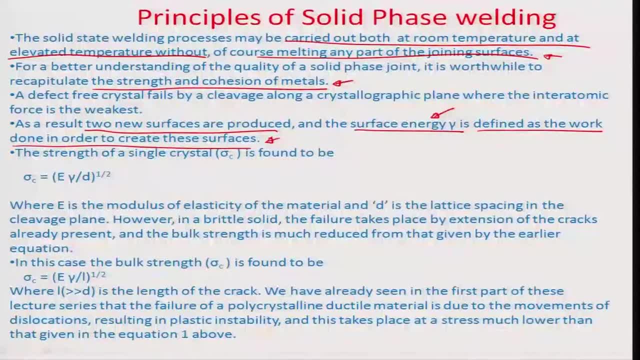 actually formulated So in a single crystal level. if you wanted to gauge what is the strength, sigma c of such a pair of surfaces created, the sigma c happens to be given by e, gamma, by d, to the power of half, where e is the modulus of elasticity of the material. 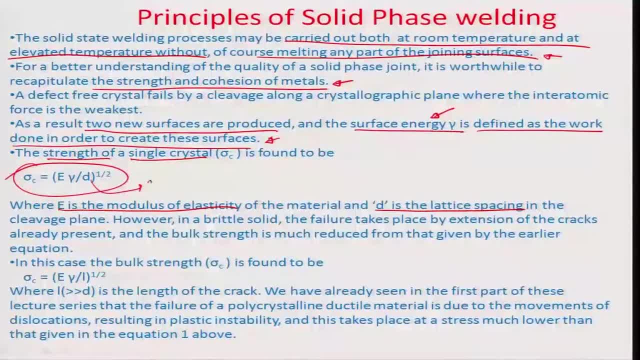 d is probably the lattice spacing. So this is actually one lattice spacing. we are talking about line materials, and particularly one lattice spacing in the cleavage plane. that is what is of concern to us, And think of it that in brittle solids the failures take. 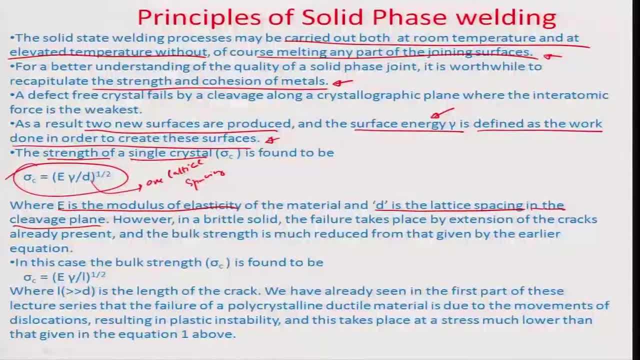 place by extension of such cracks. So therefore there is, if, supposing, some kind of a twin surface pair is created, it basically extend itself in a certain direction and we say that this is because of the crack propagation process. So therefore, the along, that particular 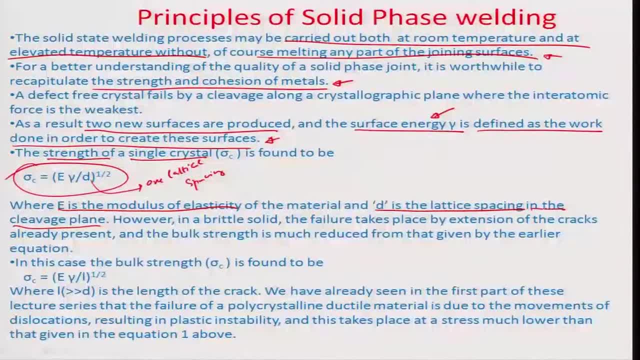 line they develop several such inter atomic spacings, where there is a new surface which starts getting created, And so there is a complete cleavage plane which is formulated, which may be more than a few lattice spacings in length. So in that, 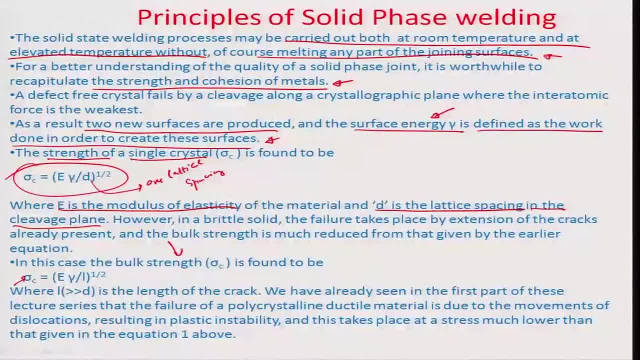 case, the sigma c which comes out, or the bulk strength of the material which comes out, is given by, again, e, gamma, by L, to the power of half, where this L, which I just told you, is much, much, much greater than one lattice spacing. So if the crack is around, let us say five different. 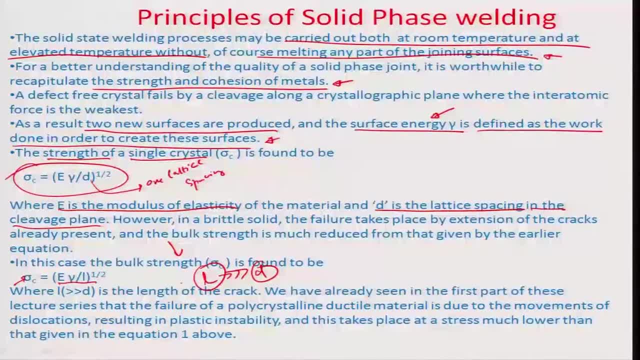 lattice spacing or even more, fifty thousand more lattice spacing. So it is a relatively larger entity in comparison to a single cleavage plane created across single crystal where the question is only of one lattice spacing. So obviously the sigma c reduces because of that. sigma c, in case of crystals is inversely. 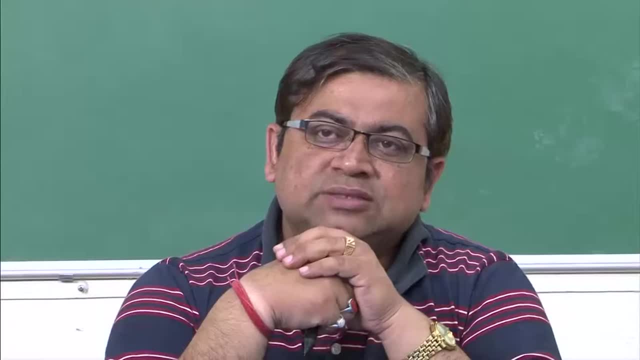 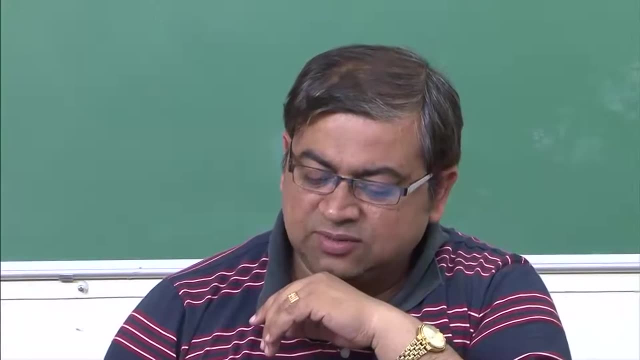 proportional to d to the power of half. in this case its L to the power of half, and L is much, much larger than d. So obviously the sigma c would be much lower in case of bulk materials than in case of crystals. So sigma c- bulk is much, much lower in comparison. 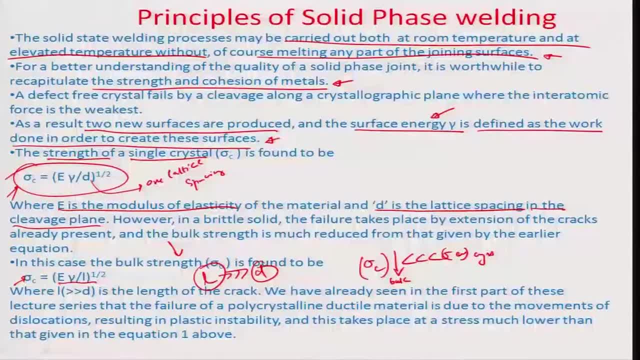 to sigma c crystals, And so that gives you a basis of why solid welding processes should happen. So we have already seen in the first part of our lecture very appropriately, that the failure of a polycrystalline ductile material is typically due to the movements of what 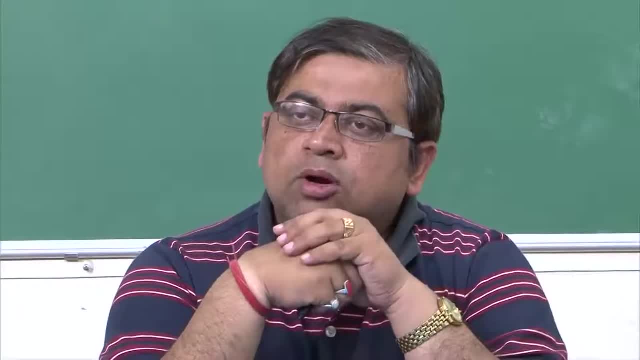 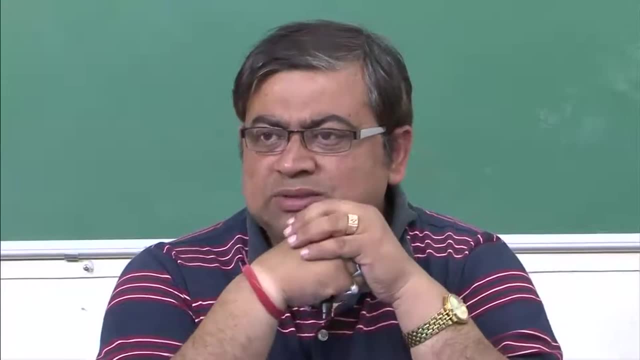 we call dislocations, which may be available over only one or two, or may be a little more size lattice planes, And this planes are sort of misfitted into the overall lattice, because of which you can say that there is a tendency of the failure of the polycrystalline material. 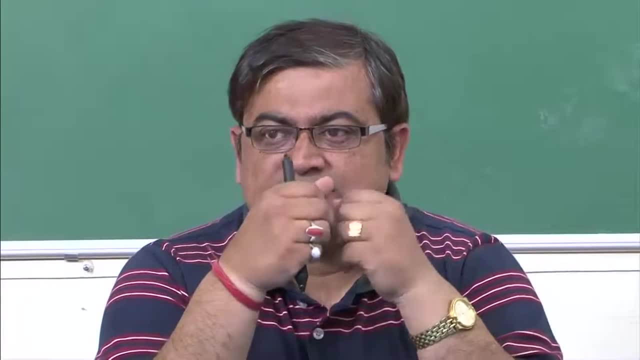 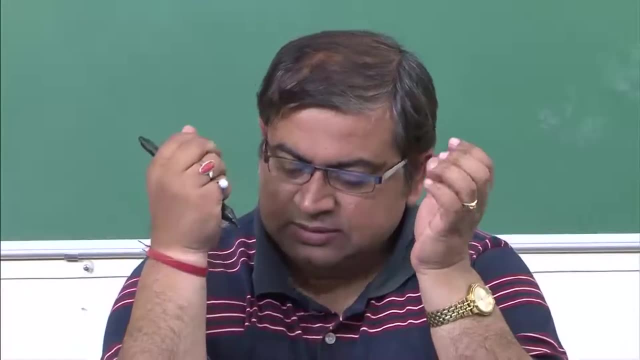 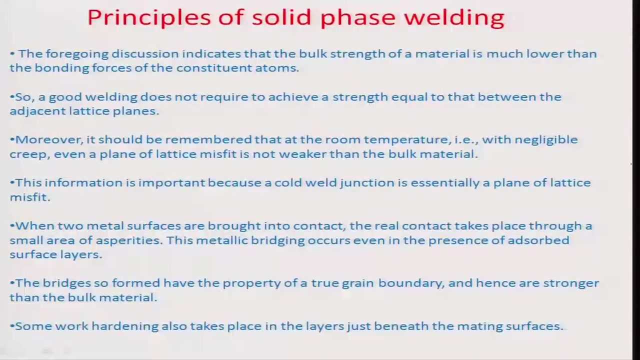 So if all the dislocations move together in certain space, there is a tendency of the energy in that region to go high, because of which the material will start breaking down and there is plastic instability because of this. So the foregoing discussion indicates that the bulk strength of the material is much. 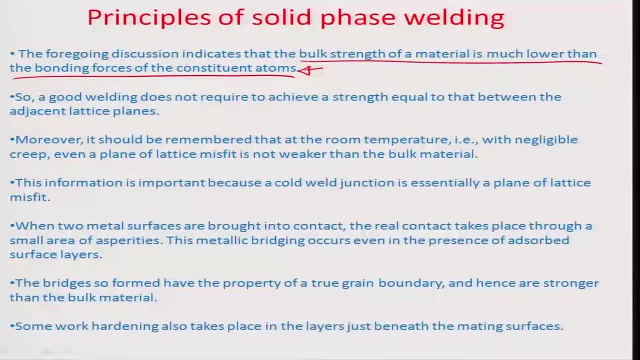 lower than the bonding force. So this is the basis of the constituent atoms. We just had an idea that in one case the total amount of ultimate yield strength, sigma c is proportional to the inverse of d to the power of half, and another l to the power of half, and l is very, very greater than d. So 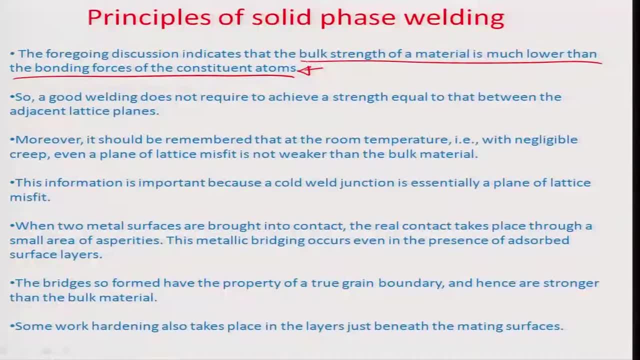 sigma c obviously is lower in value in case of a bulk material. So think of it that when we talk about a joint strength, it is about how the material would arrive at its ultimate yield strength when there is some kind of a crack or separation or something like that. 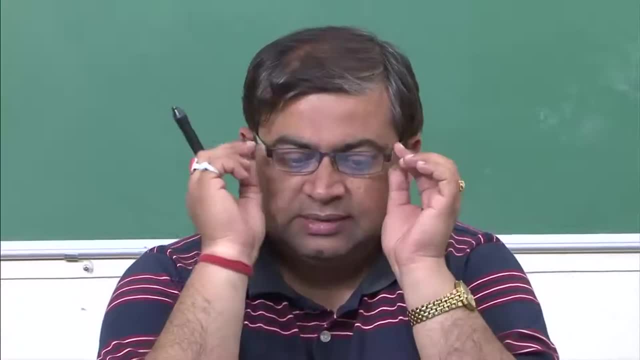 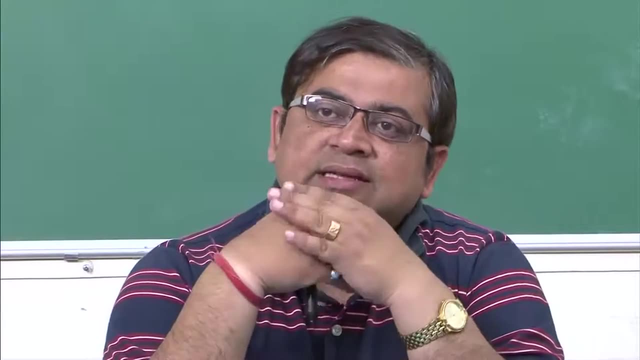 So this is the basic idea that we have to understand. So in this particular case, we are talking about a situation where we are comparing the lattice misfits because of the pressure generated between two surfaces where the distance is coming very, very close. 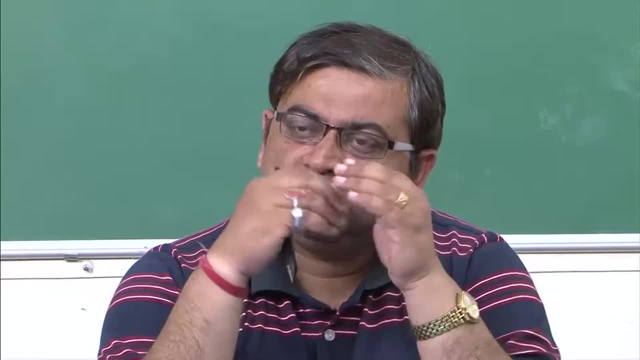 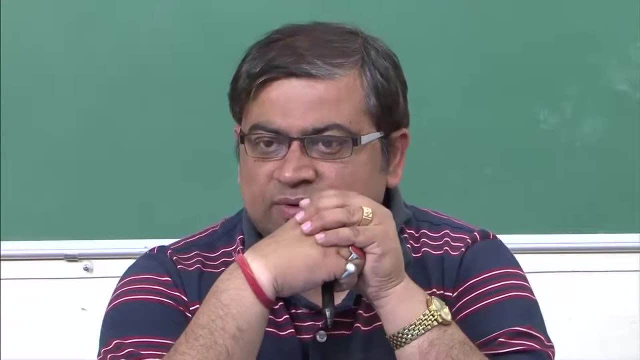 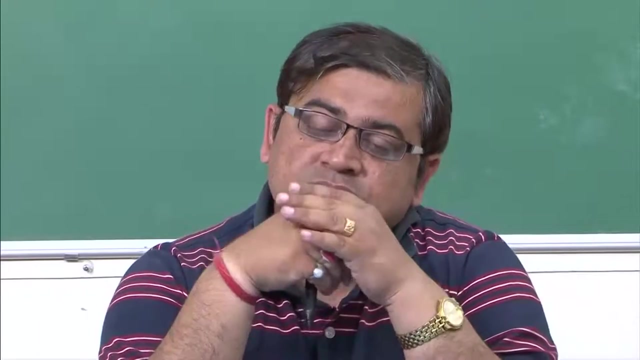 to that of a almost a grain boundary, So meaning thereby that the two surfaces that we are pressing in the solid welding is coming by a distance closer than almost one or two lattice spacing. So obviously that force would be much greater, or the yield strength in that particular region, because of that lattice misfits of. 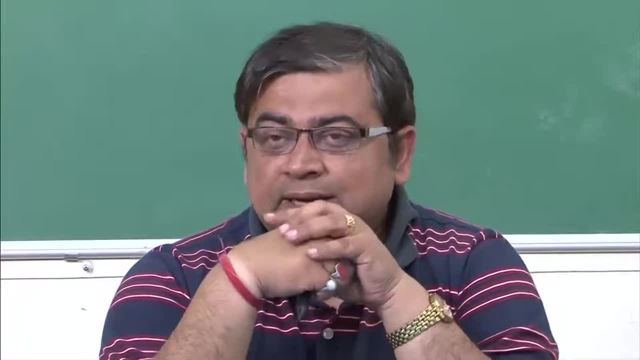 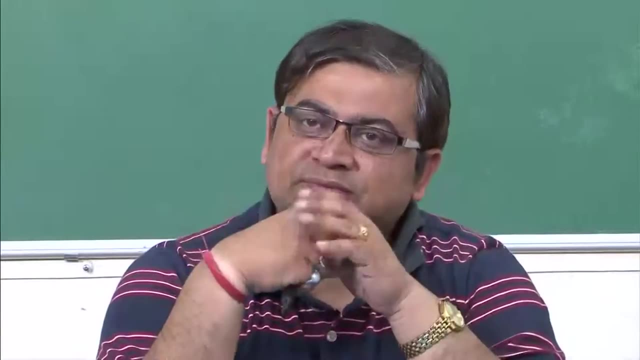 a few planes between the two surfaces would be much, much greater in comparison to the bulk strength of the material. So obviously, when in such a case, if we pull the material from both sides, the failure will take place along any other region of the bulk, but not 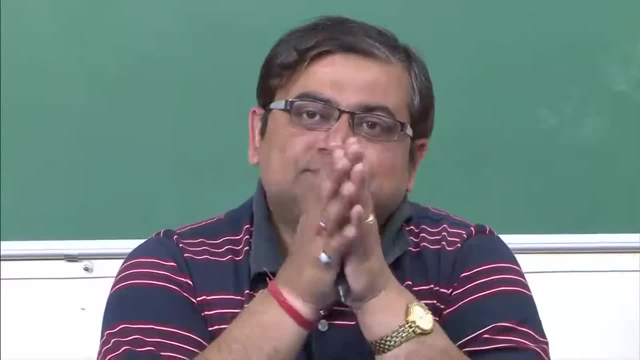 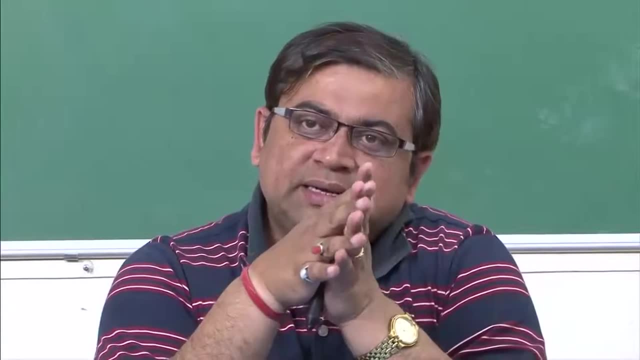 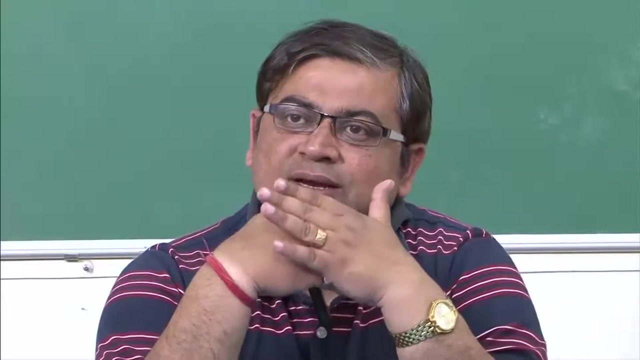 on the interface. So that is what the solid- you know- welding strength is defined as. just because in a crystalline level the ultimate yield strength increases much more in comparison to that of a bulk level, You can say that a plane of lattice misfits because of this kind of a pressure where both the surfaces come close. 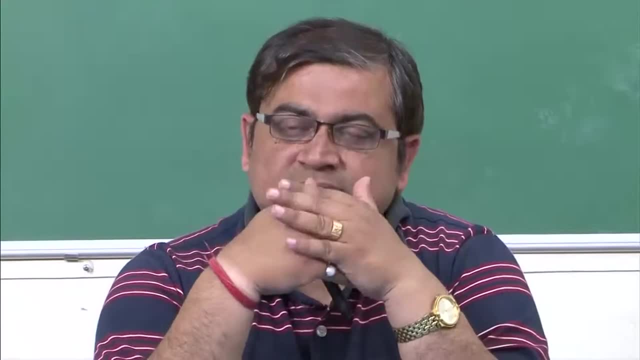 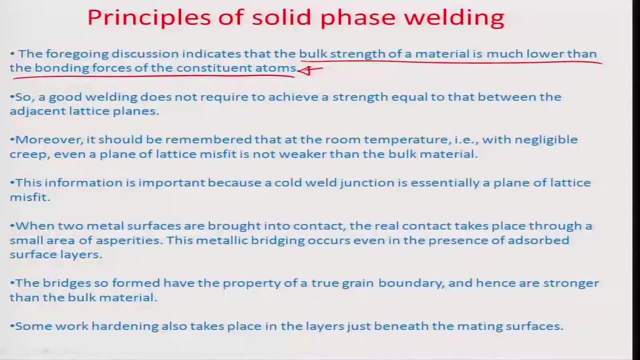 by almost like a grain, boundary thickness difference is, attains a much larger value in comparison to the overall bulk strength of the material. So a good welding does not require to achieve a strength equal to that between the adjacent lattice planes, and you must remember that at room temperature the, with negligible creep, even a plane of lattice. 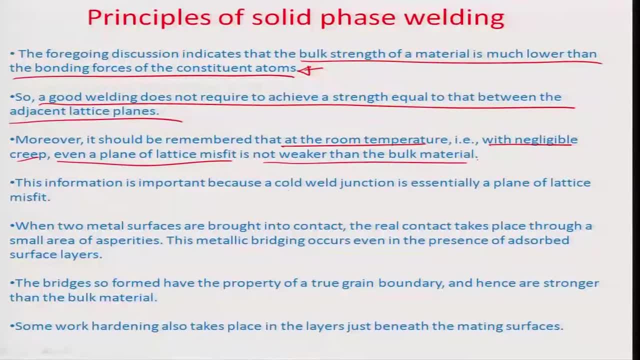 misfit is not weaker than the bulk material. So in a cold welded junction it is essentially a plane of lattice misfit which is inserted between the two mating surfaces at a huge pressure And so the contact, if we look at, between the two planes which are being brought. 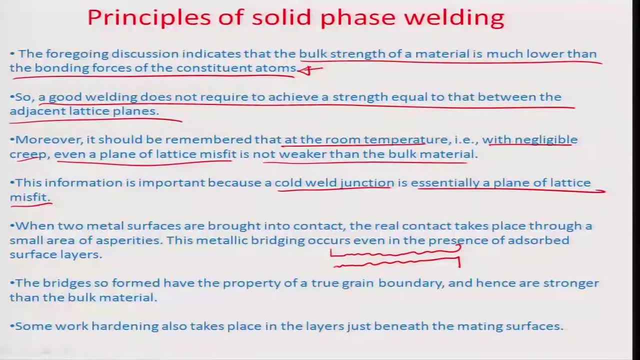 close together. Let us say we are welding these two surfaces with respect to each other, with respect to, you know, applying a Vertical pressure in between the two. So there are the small asperities between the surfaces which kind of formulate the real contact And the metallic bridging kind of. 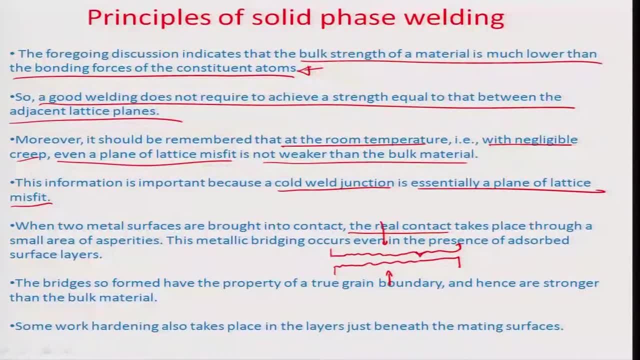 a thing happens here that supposing there is one contact which is like a hill and another which is again like a hill, So there is some kind of a when it joins each other, obviously the real area which is there, as I think I had earlier mentioned very appropriately in 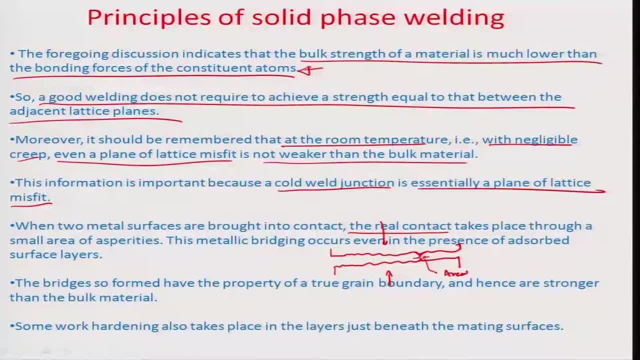 case of study of Friction is much, much smaller. So the a real smaller in comparison to the a apparent. you know, the apparent area really is that of the surface and the real area is very, very small. So in this region it is very easy to come, you know. for the overall stress, 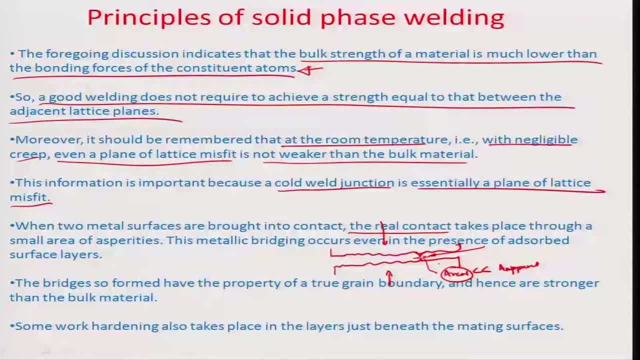 to come to the plastic deformation level And there is some kind of a deformation of these two asperities which results in a cold weld And because obviously you have brought them closer then the you know, and so that the bulk strength is kind of exceeded at that particular level And this metallic bridging 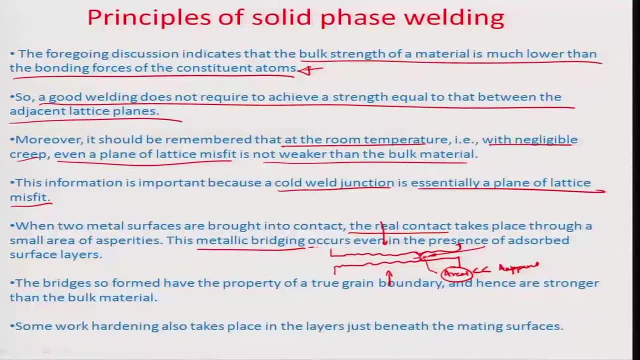 occurs even though if there are some kind of an adsorb surface layer, like an oxide or some oil, etcetera, present. still this metallic bridging occurs very well. So the bridges are so formed, have the property of a two grain boundary, and hence they are 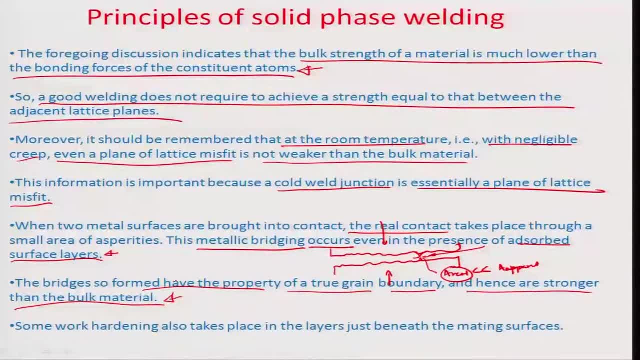 stronger than the bulk material, as I had earlier illustrated, And also there is some work hardening which takes place in the layers just beneath the mating surfaces. So overall, the weldment in this particular region, because of the work hardening underneath and the strength here, 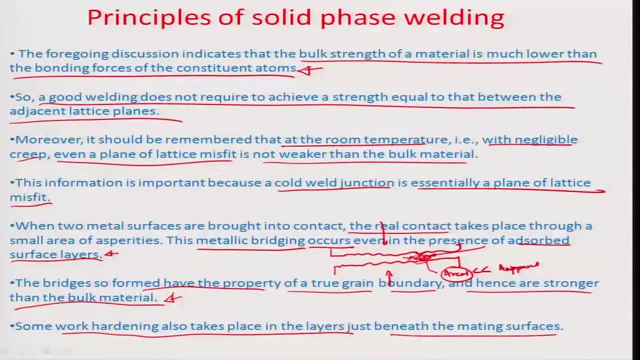 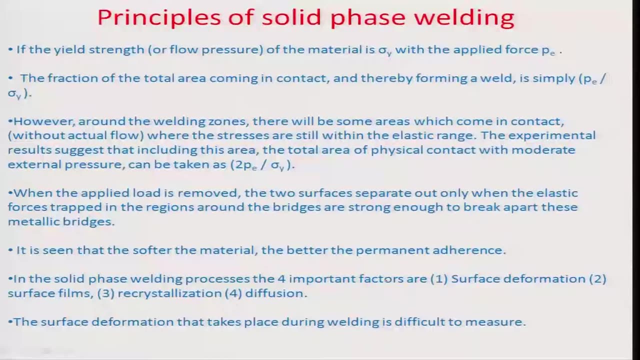 of almost single crystal becomes much larger in comparison to the bulk strength of the two materials- sigma c. So therefore it is considered to be a good weldment. So let us look at the series of events which happen in such processes. So if we considered 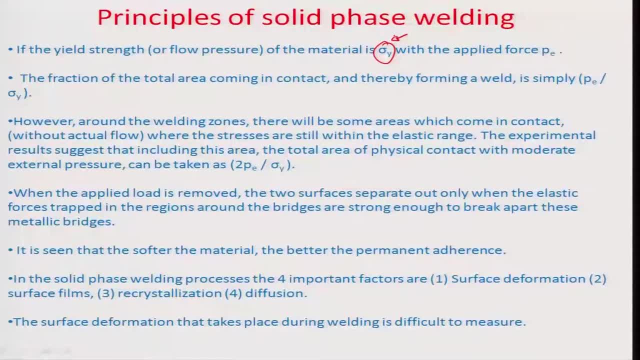 sigma y to be the bulk strength of the material, or let us say the yield strength of the material, and we apply a force P e over these two surfaces which we are bringing close to each other. So this force is P e, So obviously the fraction of the area which comes in contact. 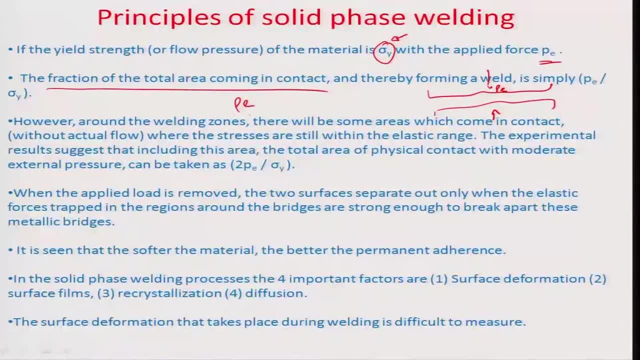 by formulating the weld can be easily given by E, by sigma y And however around the welding zones. if I look at really how this aspiriti is getting deformed, so the Aspiriti earlier was present like this, and when we have touched to the 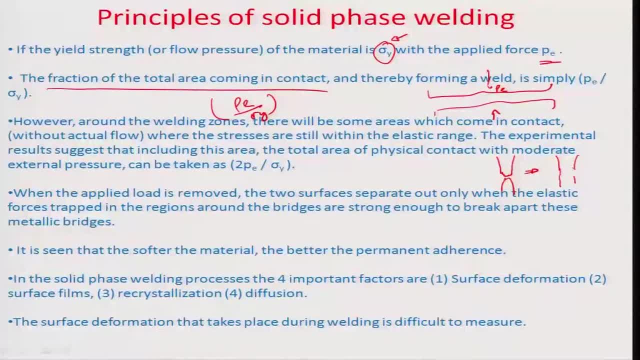 Aspiriti, the slide, deformation happens And then there is some kind of a local weld which is taken place here. So there will be some area which will come in contact without the actual flow as well, supposing there was an area just close by where the height was not so significant. 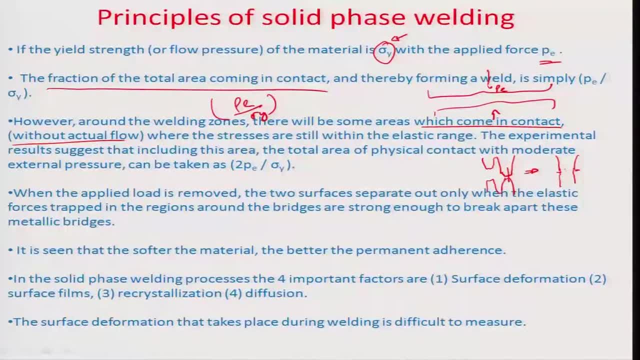 as the plastic flow would happen. So supposing these two get welded together, then it may be possible that these two just about start touching each other very close to the surface here. So there is obviously quite a bit of that area which is not so high. So that plastic 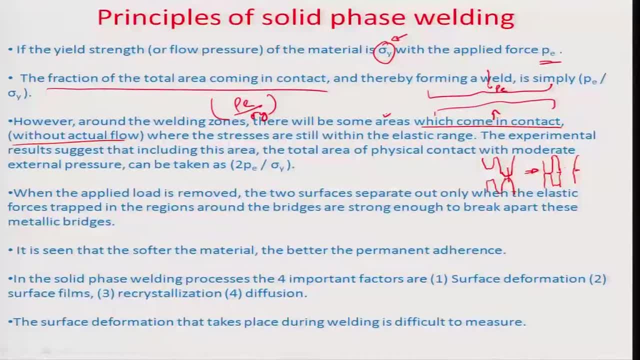 deformation would occur. but still they will touch each other when the plastic deformation may happen across some of the, let us say, top order asperities with higher heights or higher, larger heights on the on the surface. So here we can obviously say that these areas 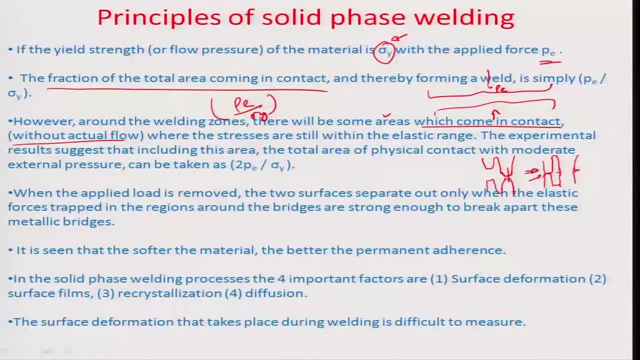 which have just come in contact without any plastic flow would still be in the elastic region. So this is a elastic region and this obviously is a plastic region, And so, really, whether the two surfaces would separate off from each other would depend on whether these 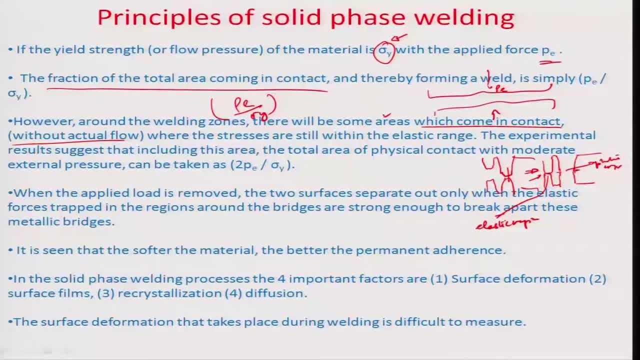 elastic forces Are greater enough to pull apart the plastic deformation and weldment which has been formulated. So if this area were very, very high, in that even obviously the surfaces would come closer. but the elastic range material, if it is not able to give sufficient amount of, So sufficient? 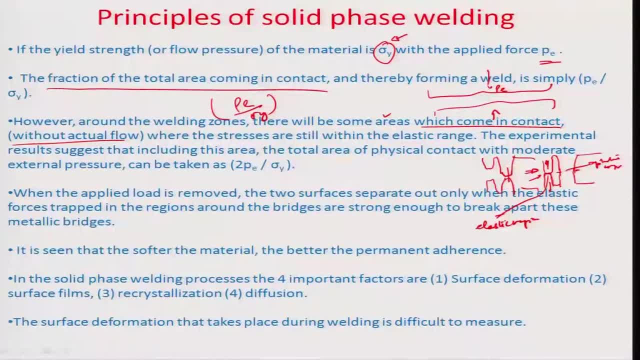 amount of recoiling force. So therefore it will not really change anything and the weldment will remain intact. So experimental results suggest that in the, you know, if you include this area, the total area of physical contact with moderate external pressure comes out to be about close to only twice this, twice p e by sigma y, right sigma. 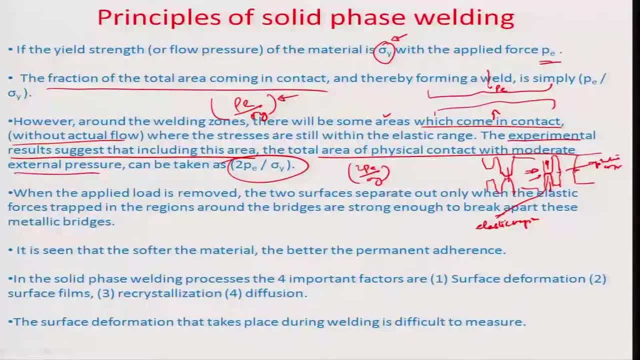 p e by sigma y was the area which was the plastically deformed asperity area, but the overall area then becomes twice p e by sigma y When the applied load is removed. the two surfaces separate out only when the elastic forces trapped in the region around the bridges are strong enough. 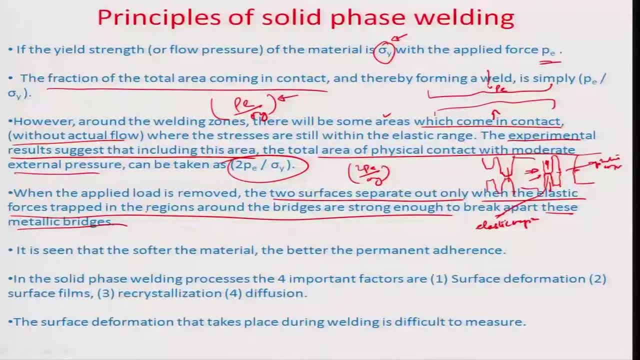 to break apart these metallic bridges. If it does not happen, the weldment would remain as such. So obviously for softer materials, where the deformation level is much, much higher, it results in a better or a permanent adherence, because more or less this elastic force may not be that critical as the number of areas which 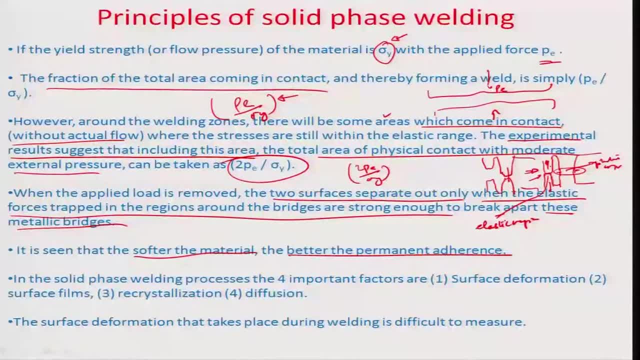 would have yielded to the plastic range would be much higher, you know, in a softer material than in a harder material. So in the solid phase welding process, four most important phenomena or factors are associated. one is obviously the surface deformation, the other is The surface films which sometimes promote or or heed, or which sometimes promote the 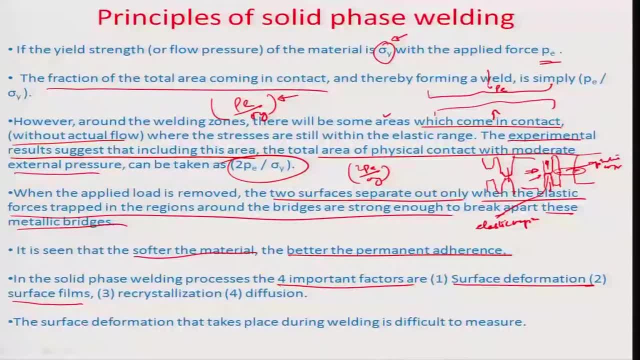 separation between these surfaces and it does not allow the contact to take place. it may be a brittle film, for example, an oxide film, where there may be some local crack propagation, which happens Where this strength aspect of bulk versus weldment, that theory may not. 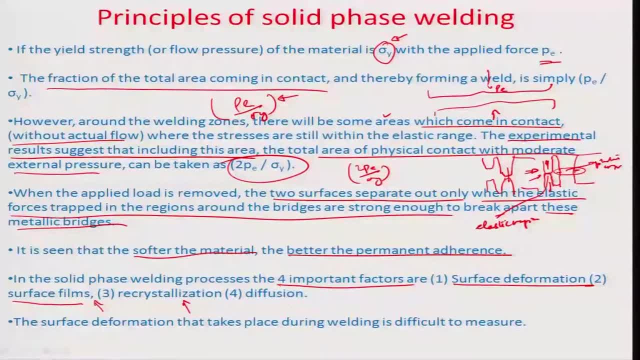 hold true anymore. and then there is also recrystallization, which may happen because physical force of pressure driven heating, of pressure driven deformation- I am sorry of the of the different grains- and then obviously diffusion, which is migration, because of concentration gradients between the two surfaces, If one surface is a higher concentration of a certain material. 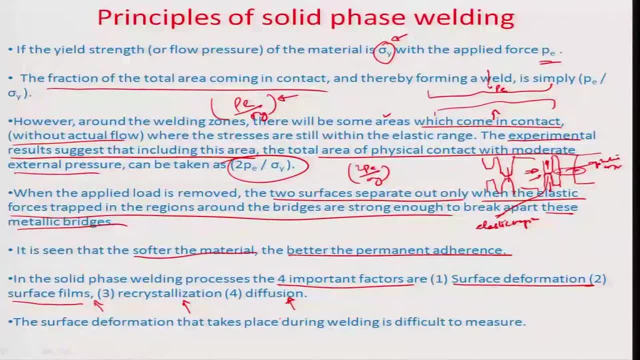 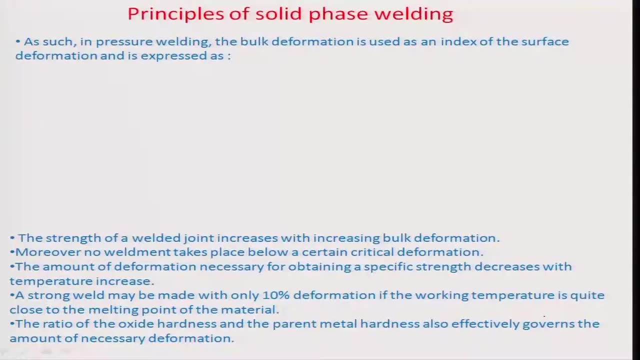 in comparison to the other. obviously there would be some diffusion through the solid state happening when it comes closer to each other. So the surface deformation that takes place during welding is quite difficult to measure, although some estimates can be brought out and, as such, in pressure welding the bulk deformation 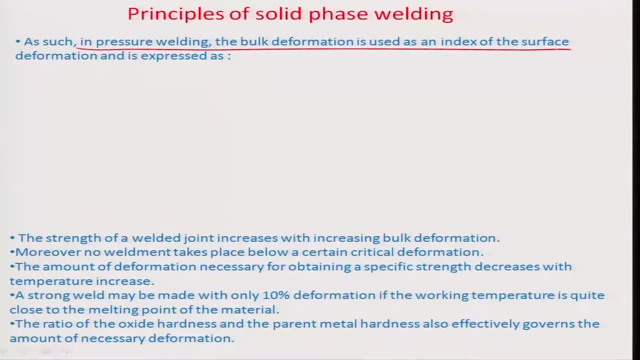 is used as an index of the surface deformation. So if I say, for a sheet of original and final thicknesses, T i and T f, I want to measure the bulk deformation, I would simply write this as T i minus T f per unit. T i expressed as a percentage and 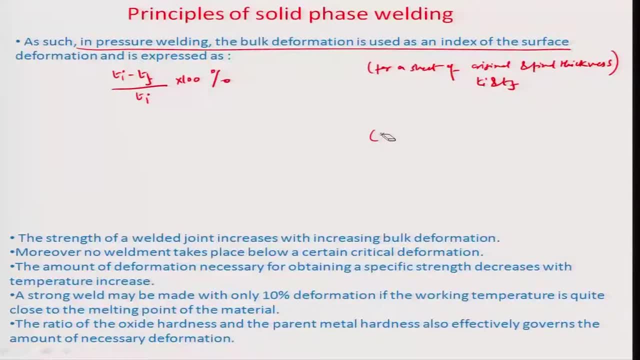 for a sheet of, or for a circular specimen of, original and final diameters, or a circular specimen of original and final diameters. So I would simply write this as T i minus T f and final diameters, T i and T f. this, respectively, would become T f square minus T i square. 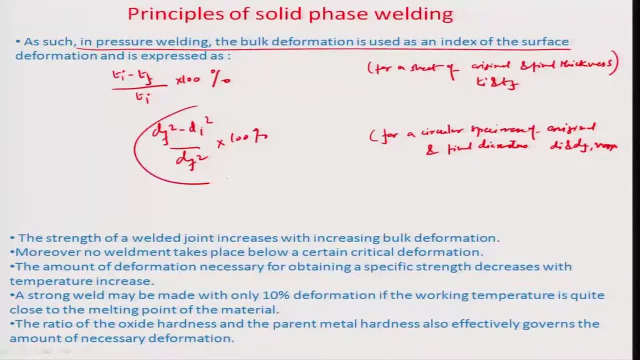 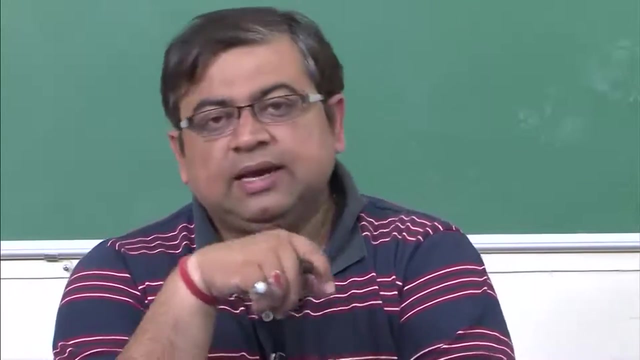 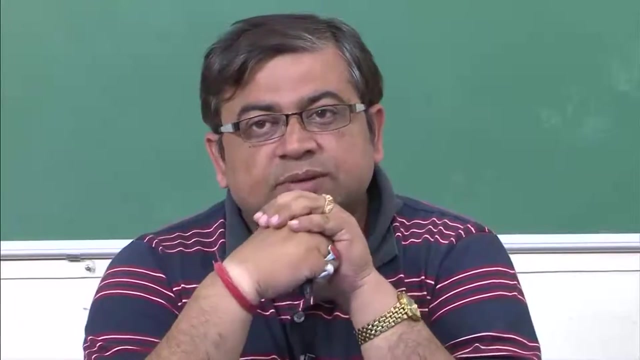 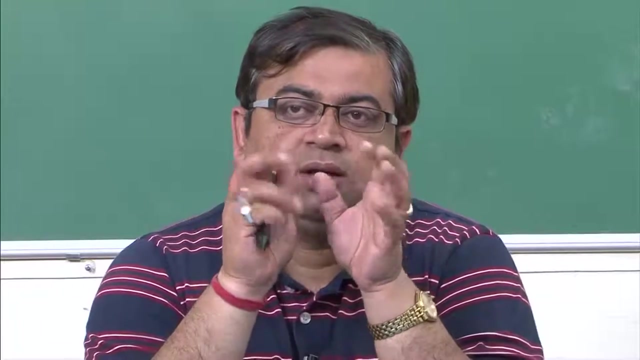 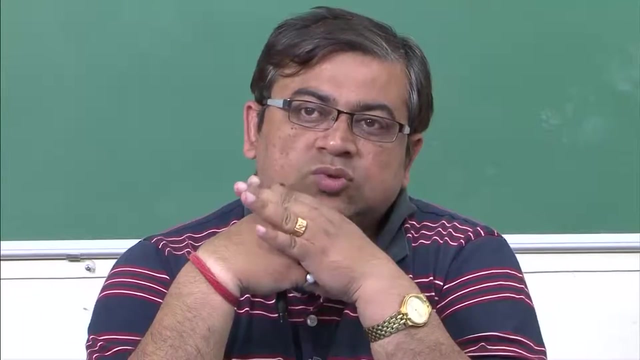 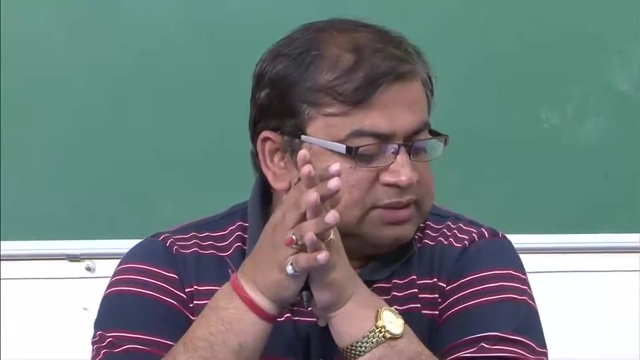 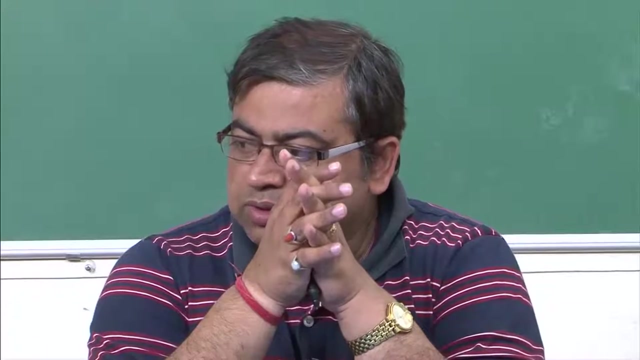 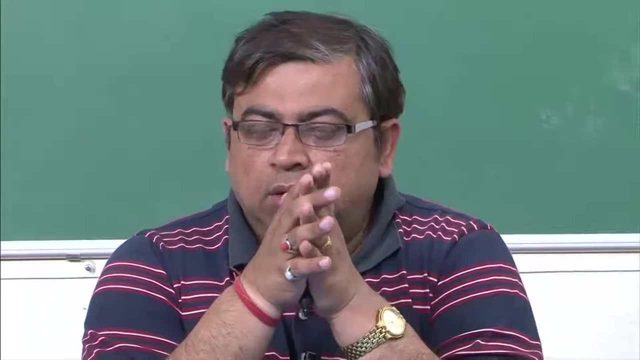 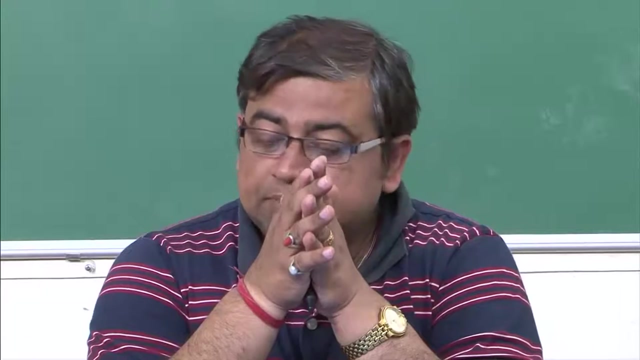 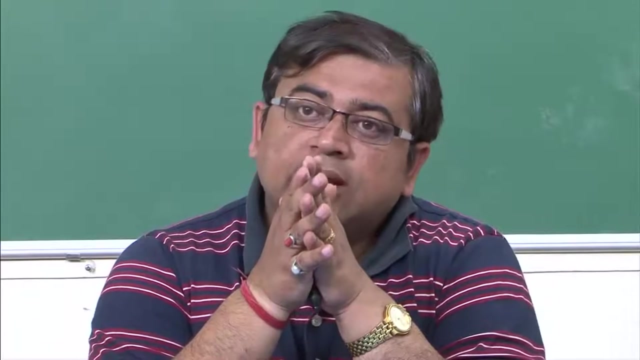 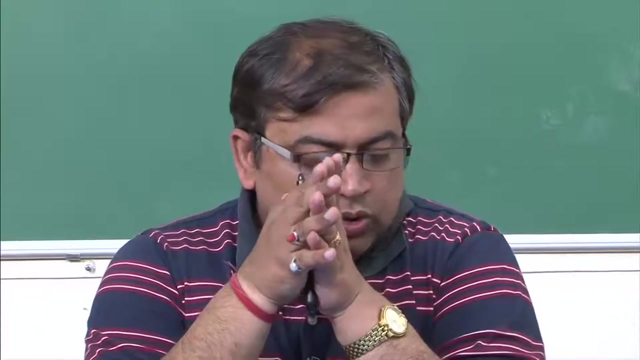 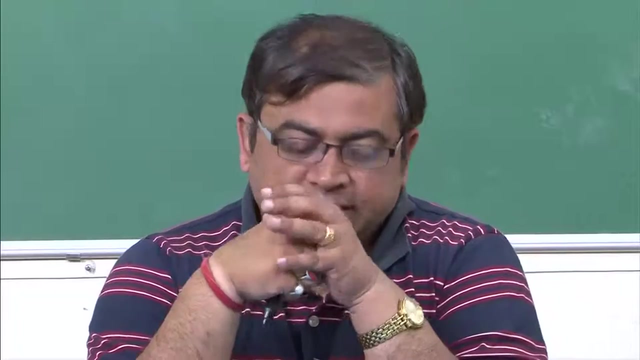 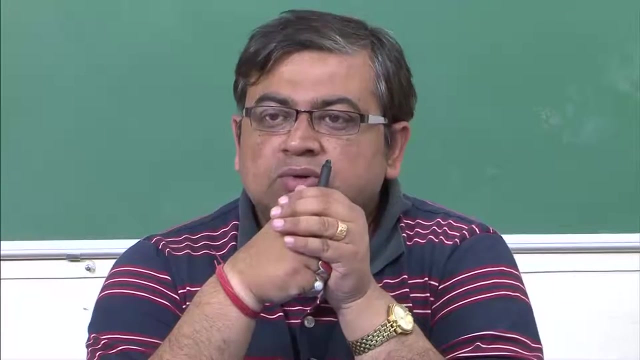 by T, f square as a percentage. So that is how you express the surface deformation of either flat sheets or round objects. But in the interest of time I would like to close this particular module. In the next module we will talk little more about just extension of whatever we have studied so far. 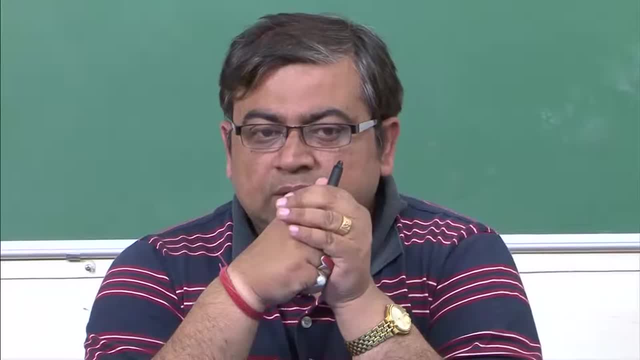 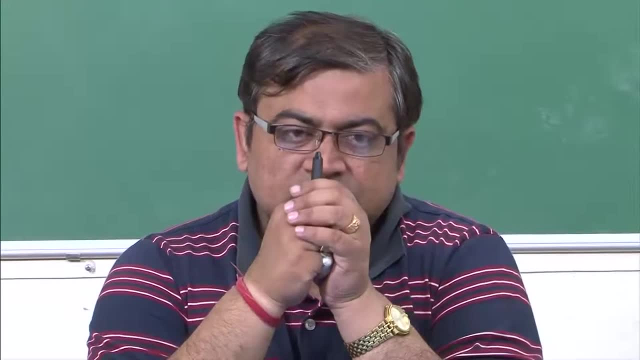 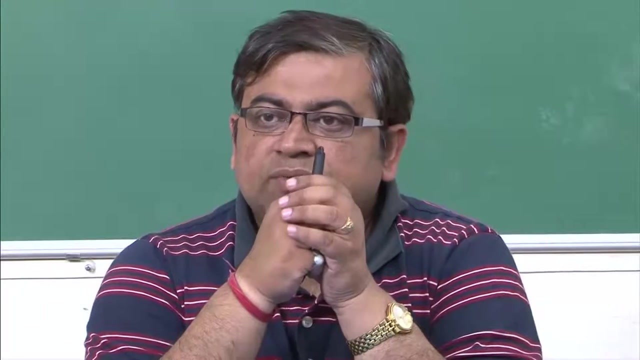 followed by studying of different sources, which would be important for us to analyze the liquid state welding particularly, And sources of heat would be something like, let us say, electrostatic arc welding. and how do we really design for a good power system, etcetera, which would do the welding properly and effectively? With this I would like to end this particular